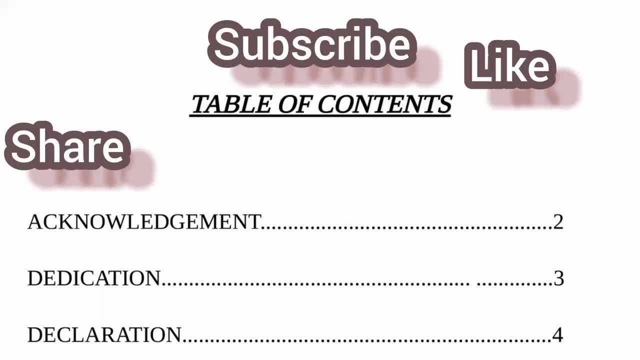 hi everyone and welcome back to my channel. okay. so sometime last year I did the video on how to write a geography field project report and I got tremendous response. a lot of the people commented asking for a sample of a PDF of the project. so I thought I would do another video of a quick outline on how. 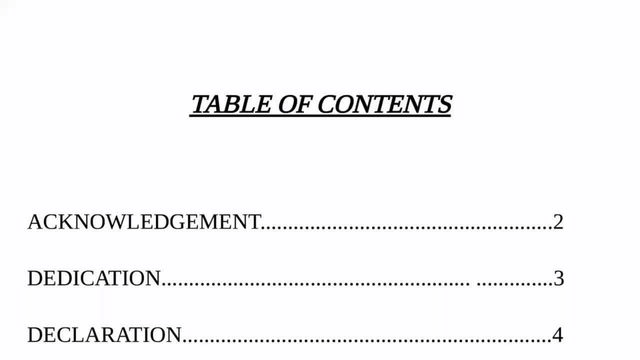 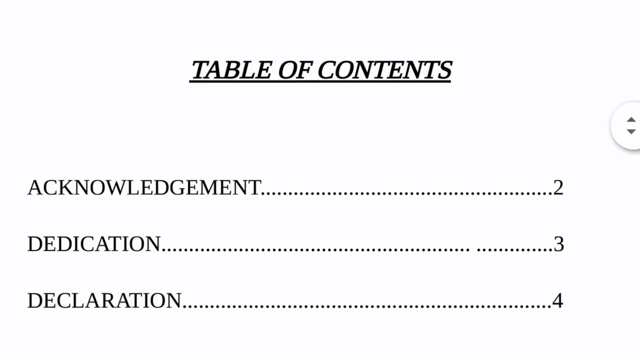 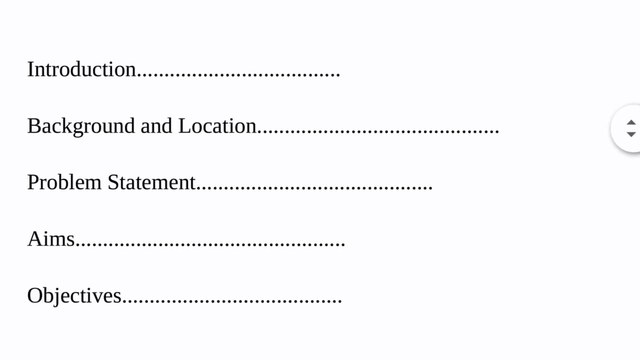 to do the project and hope this helps someone out there. so here's a quick outline that I did to help you guys out there, anyone who needs the help. okay, so it starts with a table of contents. so on the table of contents: the acknowledgement, dedication, declaration, introduction, background and location. 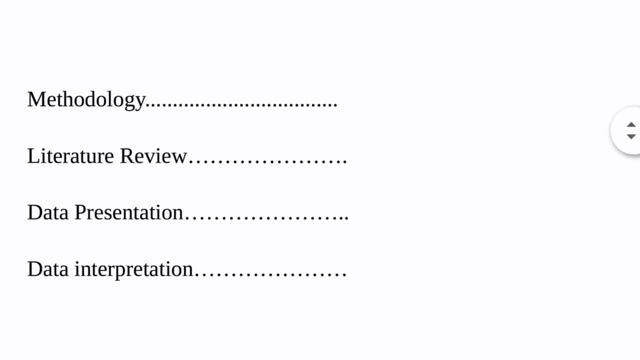 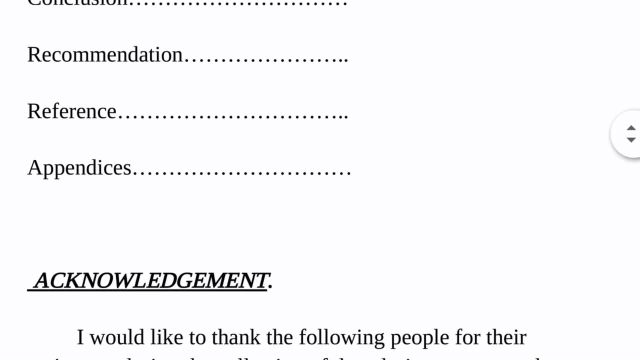 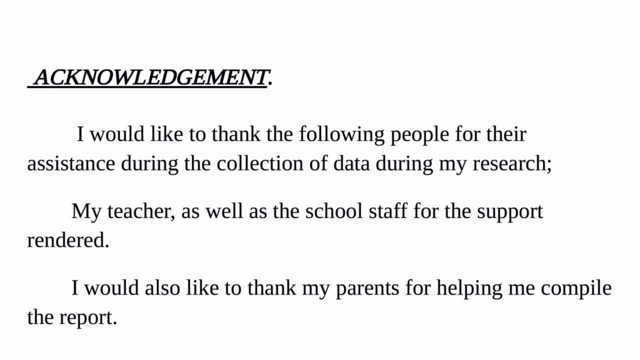 problem statement: aims, objectives, methodology, literature review, data presentation, data interpretation, problems and limitations, conclusion, recommendation, reference and appendices. okay, so we start with the introduction. oh, I mean the acknowledgement. so in the acknowledgement you simply acknowledge the people who helped you compile the report. this may. 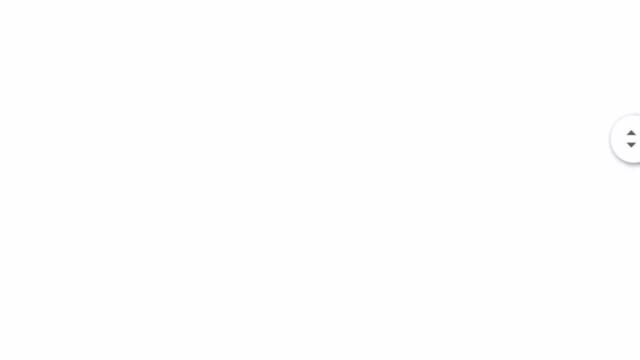 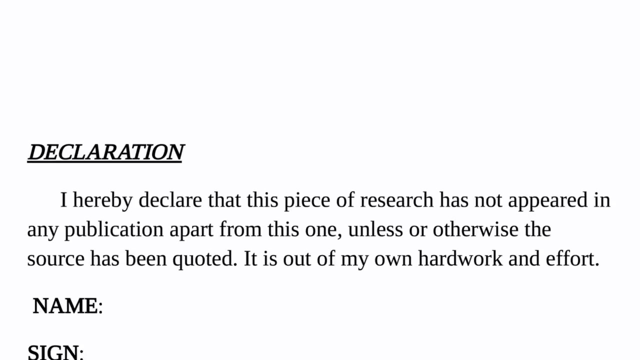 be your teachers, your parents or anyone. and then, after the acknowledgement, you move on to the dedication. of course, you also dedicate the project or this report to someone you really love. it may be your family, your parents, your friend, anyone who is special to you. and then, on the declaration, you have to declare like: 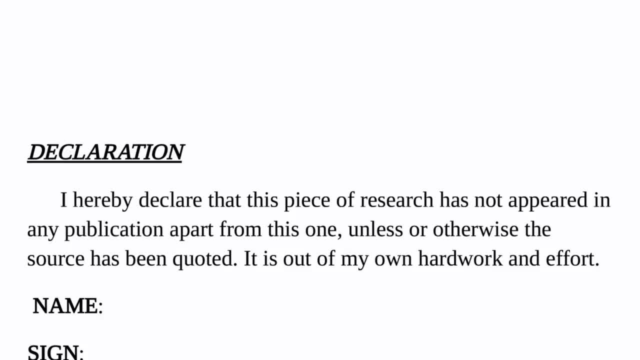 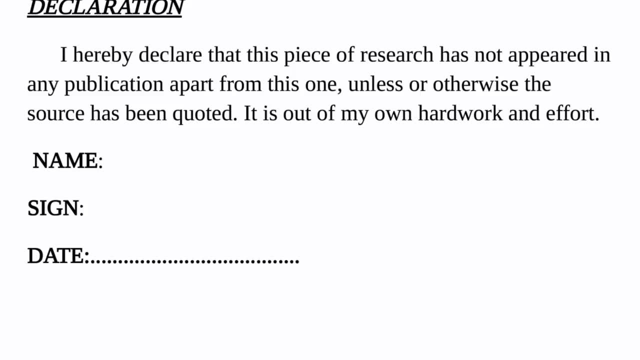 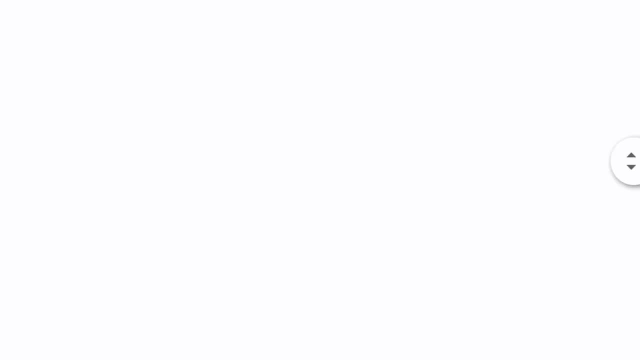 solemnly declare that you did this research on your own and it doesn't appear anywhere else. otherwise it would be like really bad if you copied it from somewhere, which would make you lose a lot of marks or even be disqualified from writing the same examination. alright, so the first chapter is the introduction of 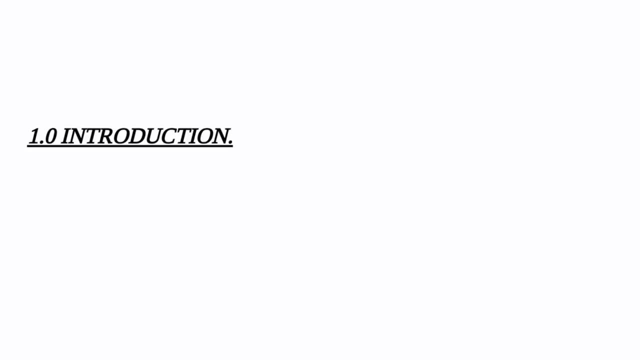 course and in the introduction, as I said previously, you write about. you just write a brief paragraph about the topic under study, its importance or significance, the problem being faced and the mitigation measures which can be put in place about a certain topic. so you can also write about how long it took you to compile 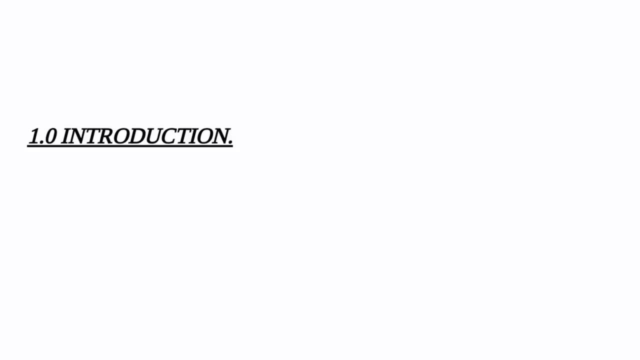 the report in the introduction. and, yeah, its impact on society, that's it, just that. and then you move on to the background. so on the background, you always be given an area of study, of course. so under the background, you can write quick, a quick history about the area under study, the area under study that you've 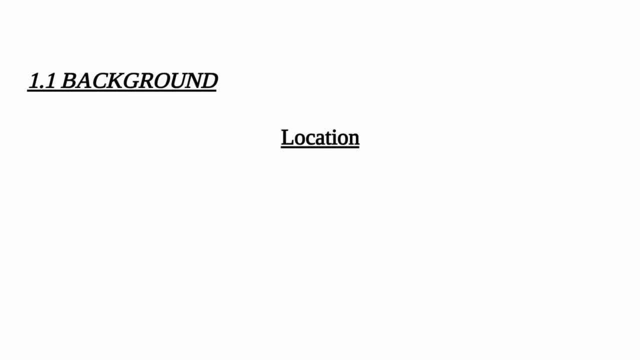 been given and simply indicate when the place was founded or where the place is located, of course, the location. you can put it under the map, and the map should be clear, it should have a compass showing all the directions, of course. and then we move on to the statement of the problem or problem statement. so, um, a problem statement, you can simply define. 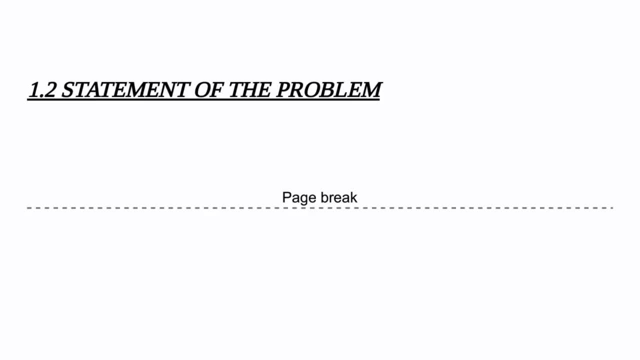 the key term um. let's say, for example, you are researching on horticulture, of course, so um, you can just define what horticulture is. or you can just briefly define what horticulture is and um, statewide it will be important to study about it. yeah, that's it. and then, on the m, 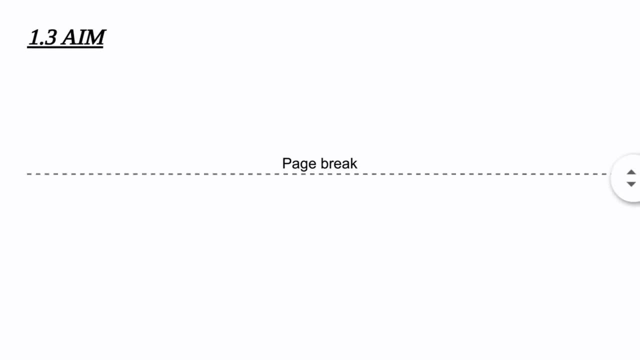 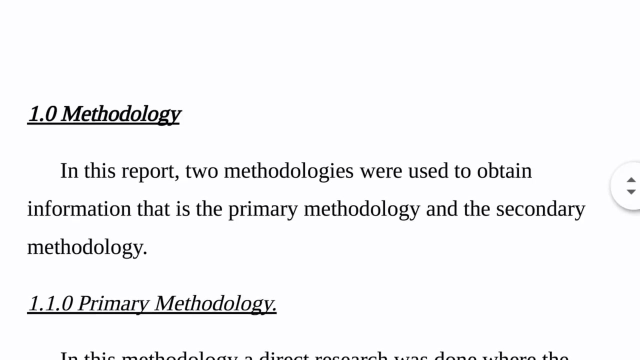 on the m, you just write about the aims of your report, what you aim to accomplish from your report, and on the objectives. on the objectives, you write about what the study intends or plans to do on a certain topic which is given. then you move on to the methodology, and on the methodology, you simply write about the methods you use to. 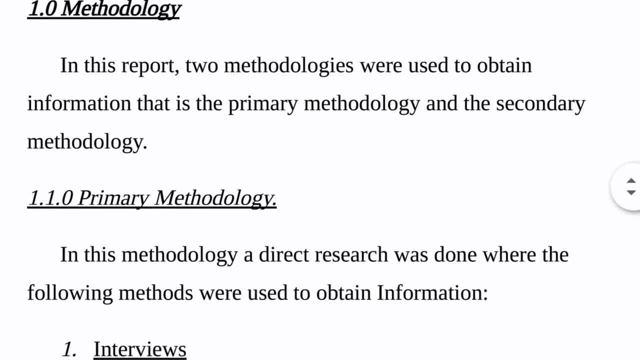 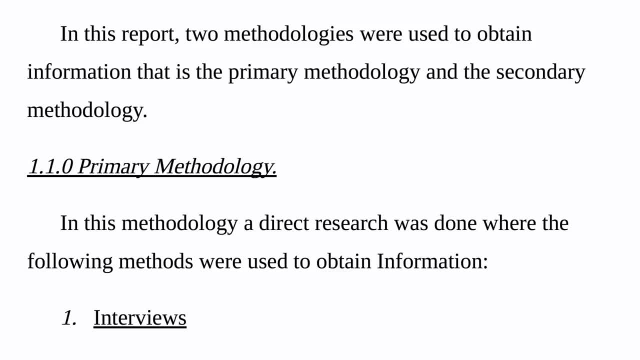 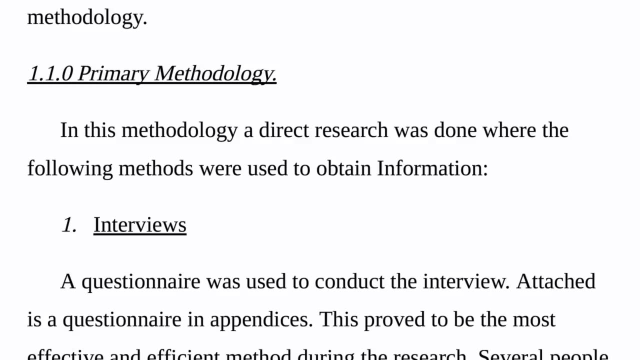 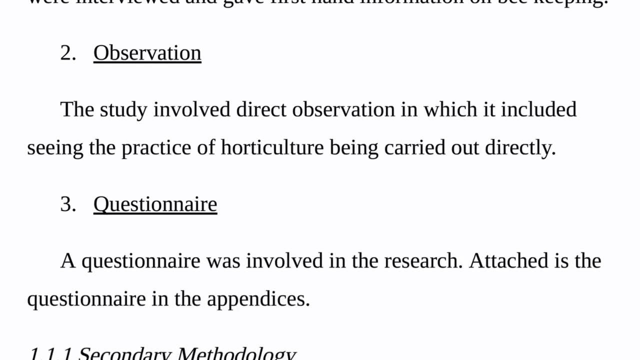 obtain your information um. so mainly the two types of methodologies, of course, which are there, which i mentioned in the previous video, are the primary methodology and the secondary methodology. in the primary methodology, information is mainly gotten in form of questionnaires, interviews, observation um of the area under study. 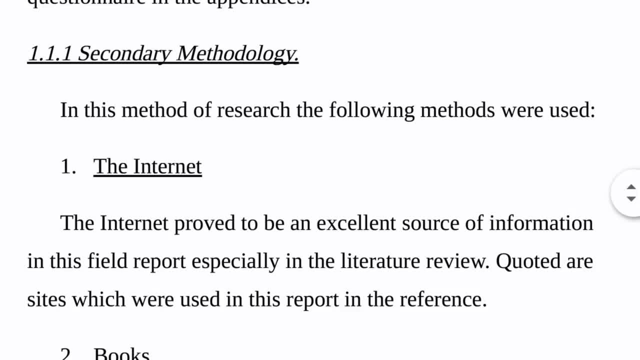 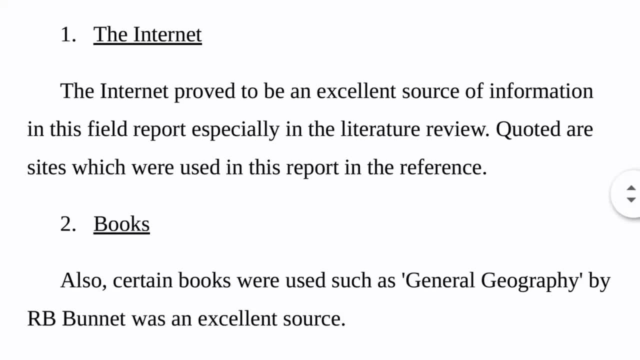 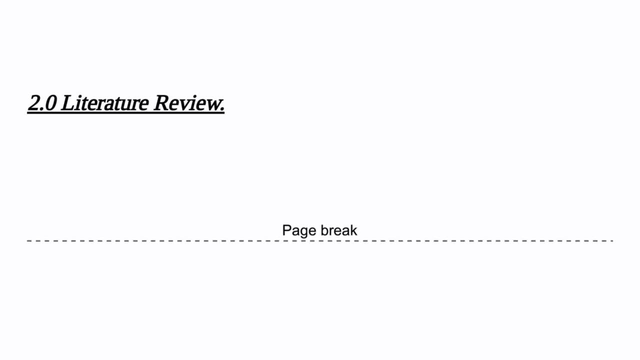 then on the secondary methodology, it's also easy. you obtain the information from the internet, the media. yeah, simply that. then, um, you move on to the literature review. so under the literature review, you write about past studies which were done on the topic and that Gö, and what can be done to improve them. 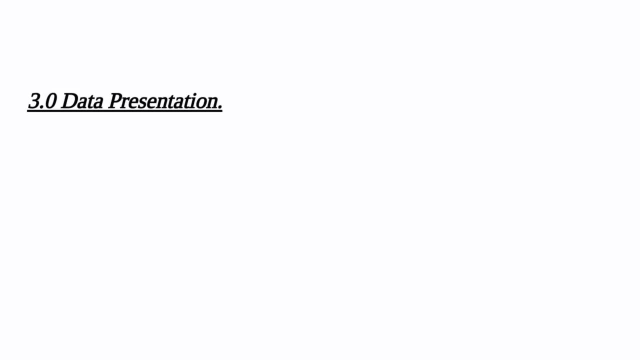 Yeah, that's it. Then, on the data presentation, you simply present the data you researched during your field trip or your field research in form of pie charts, tables and graphs, et cetera, and further interpret them in form of words. 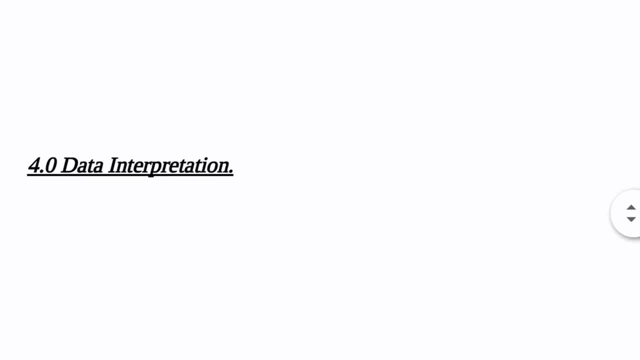 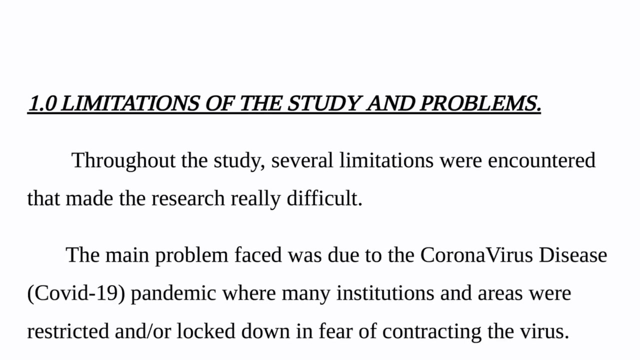 Yeah. Or you interpret them in form of words on the part for data interpretation, where you write more about the data you obtained: Yeah, Then the limitations of the study and problems. you just write the problems you really faced during your research. For example, I wrote a brief. 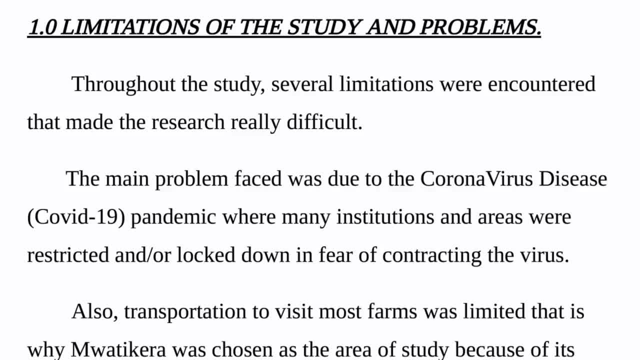 a typical example Of how you can write your problem statement. You can, for example, the main problem which was faced last year, for example, and this year- part of this year- is due to the pandemic. The research: some centers are still closed for research. 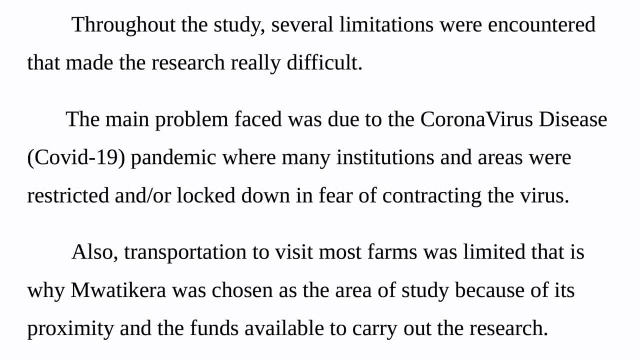 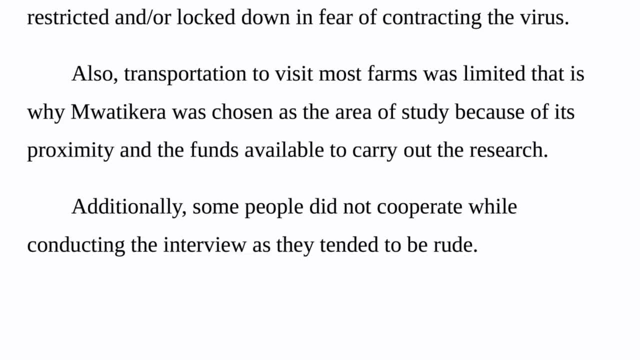 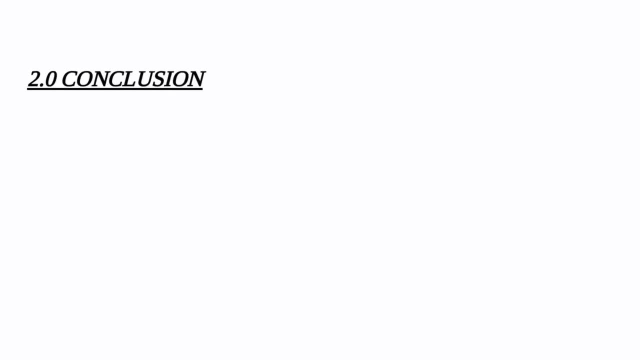 So you can write about how COVID is affecting you or how transport affected you during your research and how maybe people were not cooperative during your interviews and stuff, And then you write the conclusion. On the conclusion, you just write your opinion about the whole research.